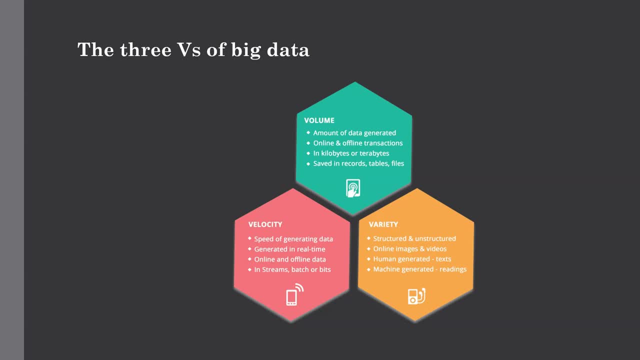 before Now we will discuss the three v's of big data. So those three v's are volume, velocity and variety. So the volume means the amount of data really matters. So with big data you'll have to process a very huge volume of load density and a unstructured data, So this can be an unknown value. 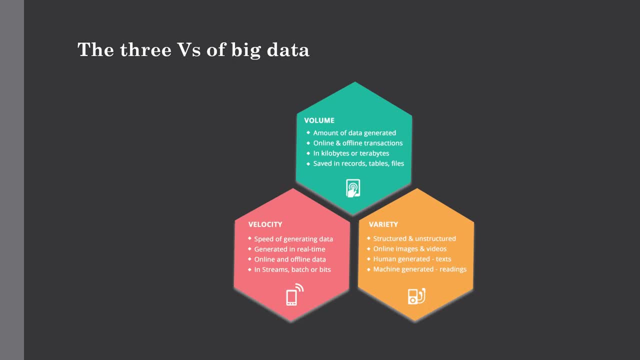 such as Twitter feeds, click streams on web pages or a mobile app or some sensor based equipment. So for some organization this might be some gigabytes or terabytes of data, but for others it could be a hundreds of petabytes of data. So the volume is a very essential part of big data. The next one is velocity. So it is. 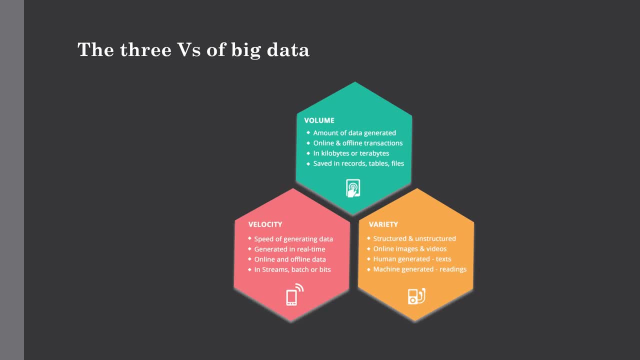 rate at which the data is received and acted upon. So normally the highest velocity of data streams are directly generated by the data stream. So this is the rate at which the data is received and directly into memory versus being written to the disk. So some internet based smart products will. 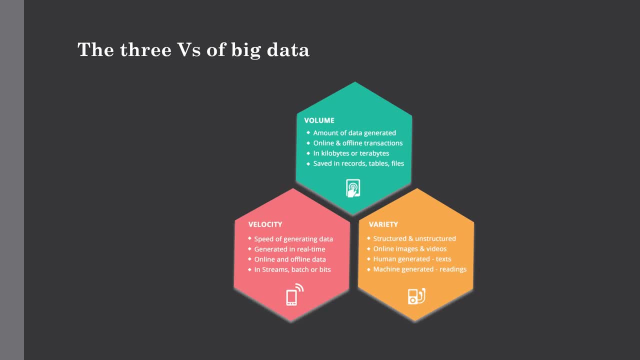 operate in real time and it will require the real time evaluation and action on that data. And the third v is variety. So it refers to the many data types that are available nowadays. So traditional data types were structured and can fit neatly in a relational database. But with the rise of big data, 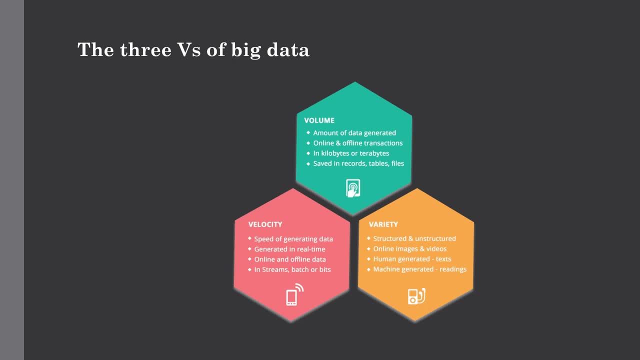 it comes down to the amount of data that is received and the amount of data that is received. So it comes in unstructured data types as well as semi-structured data types, such as text, audios and videos, which require some additional pre-processing and cleaning the data to derive some meaning out. 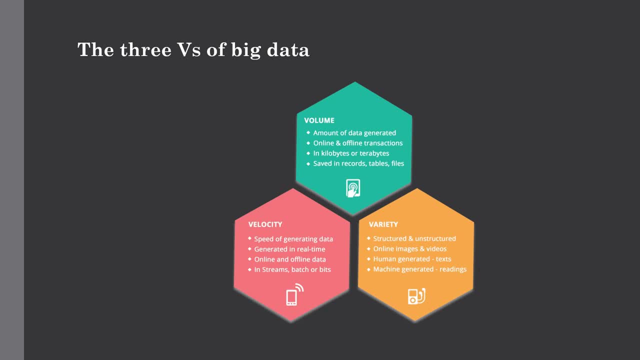 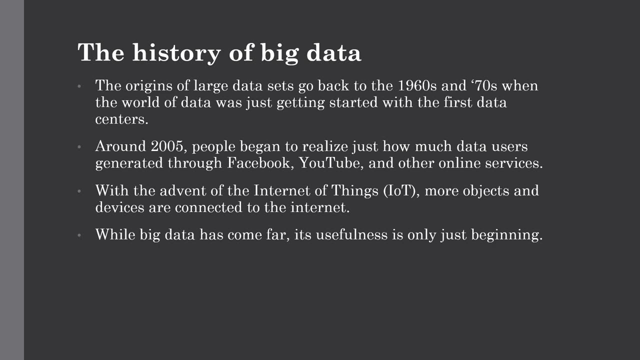